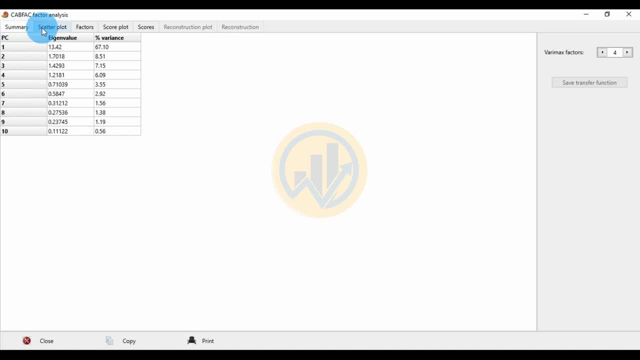 variations: the 0.56. then next one's menu for the scatter plot. this is a scatter plot for the factor analysis is: this is factor one and this is a factor two. the factor one is a plus, the factor two is a minus. the range: the. before the click the row label for the the dot the click the row label, checkbox this. 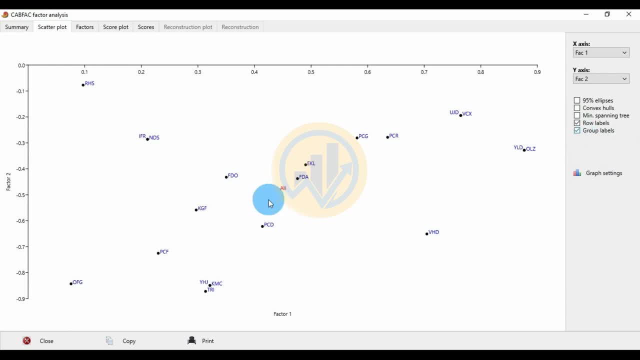 is a location, the label, then the group label, the cell, the all, the group label for all, and there is a clear 95 itself of the click. the 95 cover the whole. the locations, okay, the first one for the, the present in them, factor variations, the next one for the factor range, the factor one, factor two, factor three. 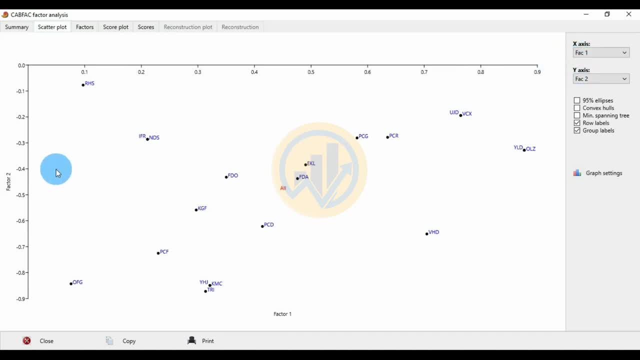 this is a factor one. uh, xs is a factor one. the xs, xs, ys is a factor two. if you change to, x is a factor three, this is a factor three and this is a factor one. then x change to factor four. this is here factor four and this is a factor two. first we sell the factor one and the factor two compared for the. 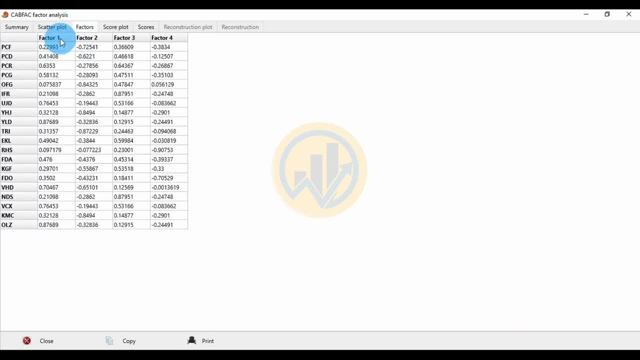 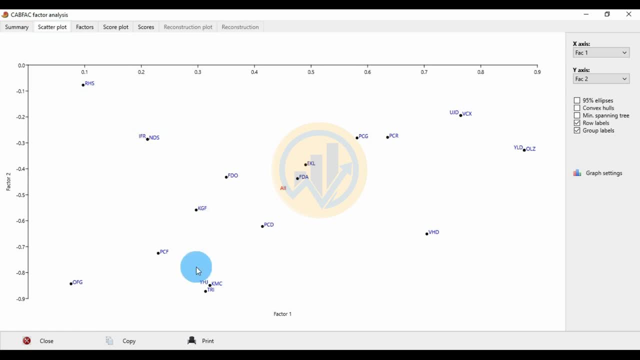 species distributions. the factor of the range for the next one step, the first one for the factor one. this is a factor two. that p a, the first select for the location. pcf, the pcf represented in the the. this is a pc, uh, pcf. the percentage here for the value for the factor one. 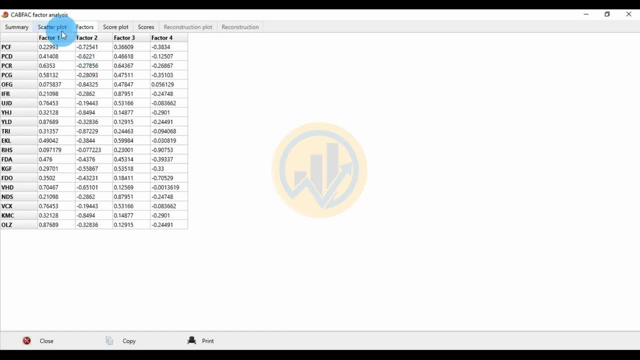 the 0.22 on factor 2 minus set 0.72. the 0.22, then factor 2: 0.72. the next one for the gf, OGF, ogf: 7.22. OGF factor 1 percentage value for the 0.075837, at same time the factor 2 value 0.-0.84325. 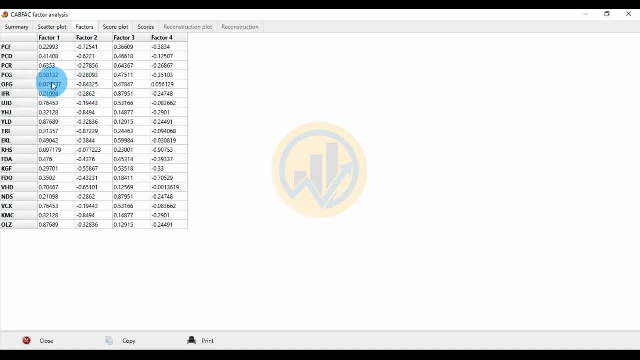 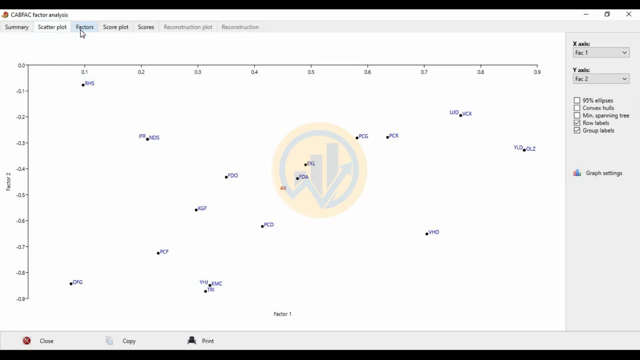 okay, this is a OGF. the OGF factor 1 is a 0.075. the OGF 0.075 is a factor, the positive and at the same time the negative for the 0.84, the minus 0.80 for the OGF, the all the. 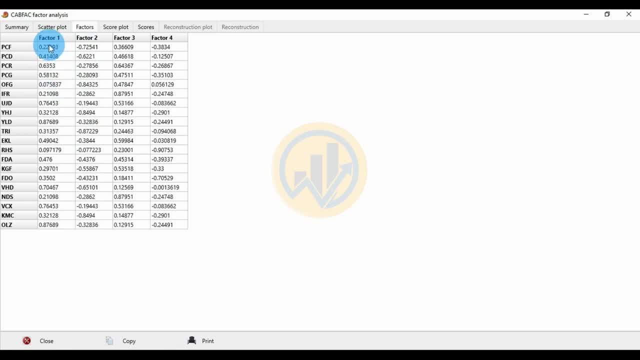 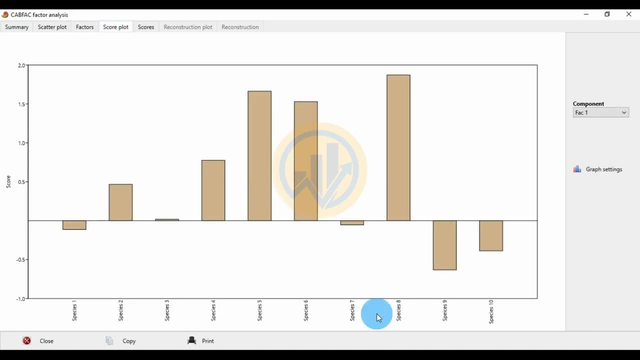 location, the value presented and the, the third column for the factor one, factor two, factor three and factor four. what are the locations then? next one for this score: blood, the score part presented, the tens, BTS. The common for the four factors is a factor 1, factor 2, factor 3, factor 4: change is factor. 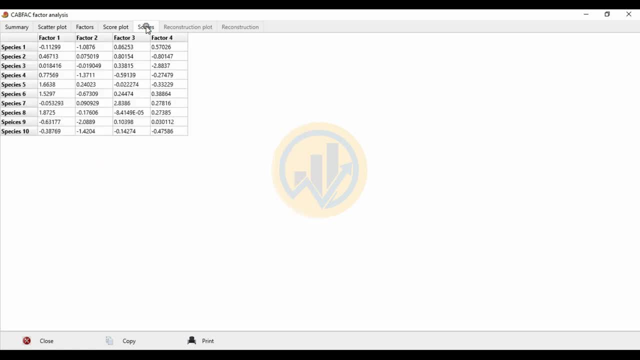 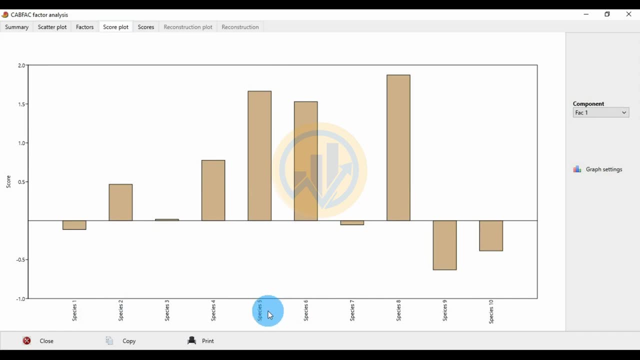 one, two, three, four, the score value presented. the next one column for the score: Valley, factor 1. factor 2. factor 3. factor 4, past, which is the factor one, The factor on the matter negatively presented for the species, one species, seven, nine and ten, the factor one. 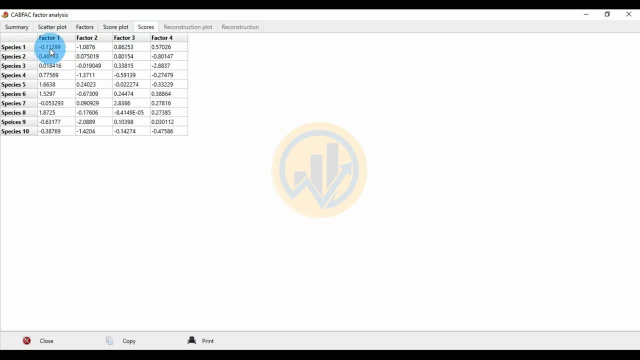 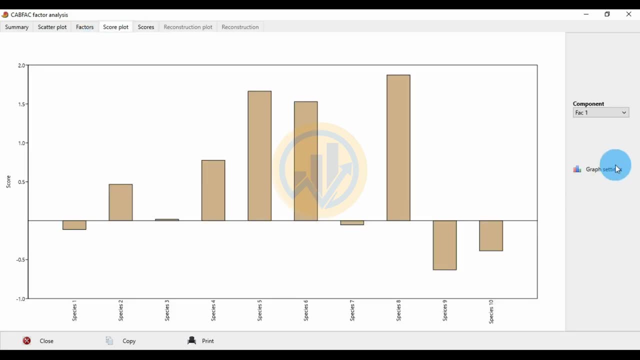 the factor one is negative. presented value for the factor one: species one, species seven and the species nine ten. the next one for the compound of the factor two: the factor two: the most of the species presented in the negative: the species one, four, six, eight, nine and ten. okay, the most of the. 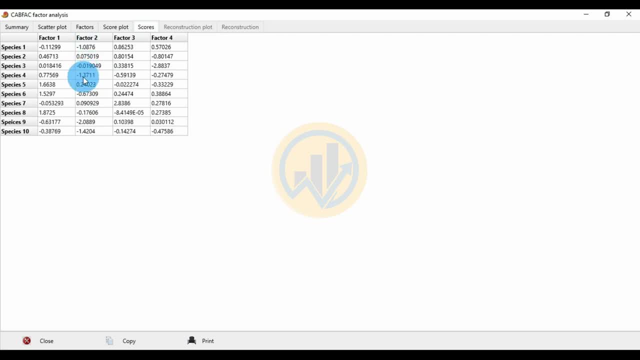 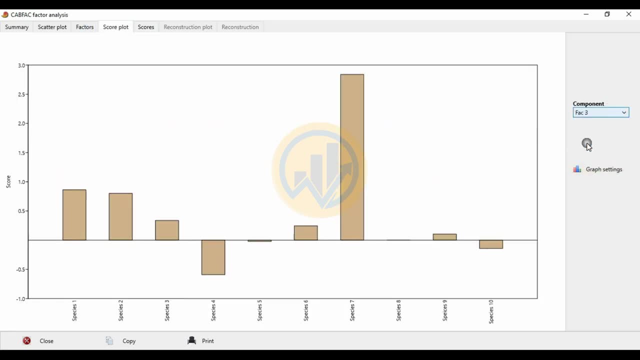 species presented in the negative for the species: one species, three species, four species, six, eight, nine, ten and the third one. for the factor three: the factor three: only the three species presented the negative and seven species presented in the positive value, the next to the compound for the: 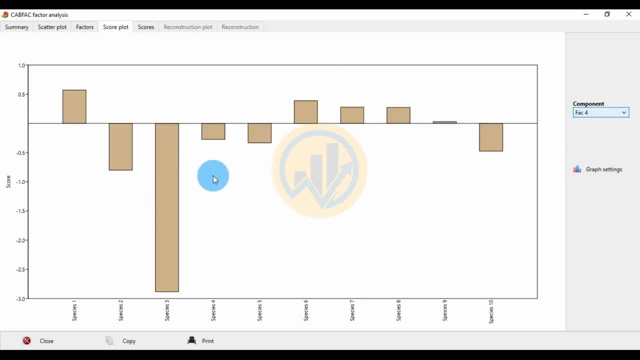 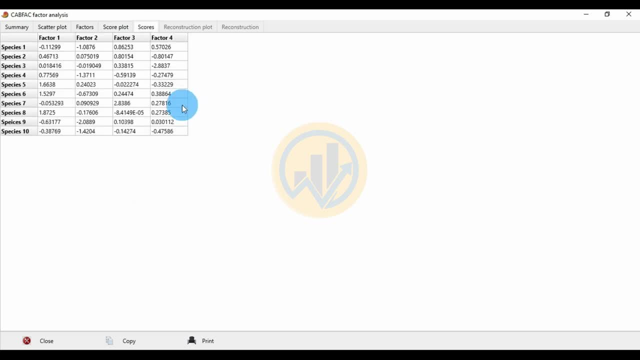 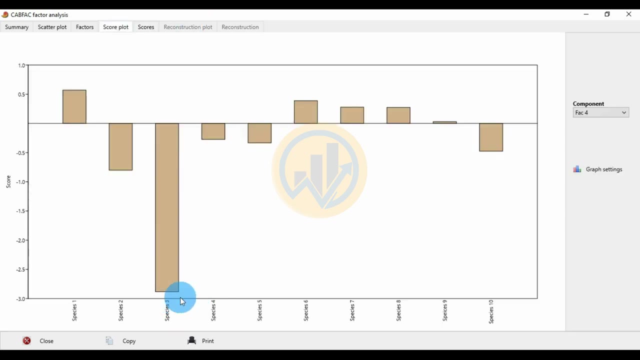 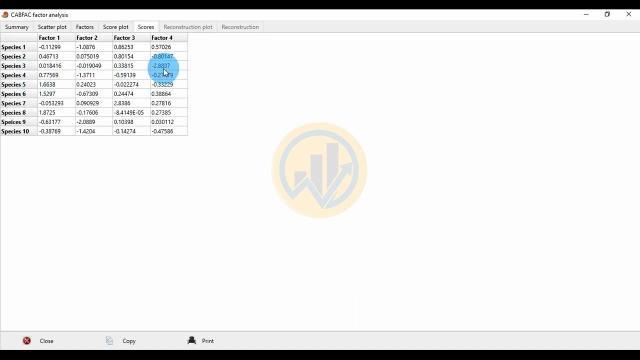 factor four: the factor four, the presented in the four five species in the negative value, the highest, the value for the species in the factor four, the highest in the species four for the minus 0.77. okay then, okay, species three: highest: the species three minus two. point double eight, three, seven: the highest negative factor presented in: 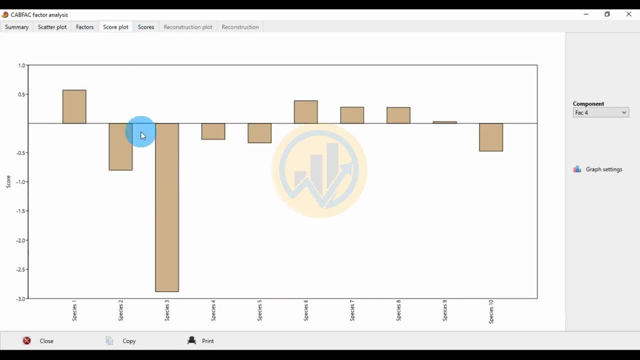 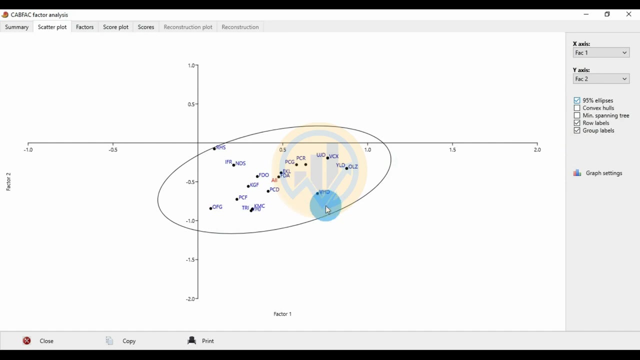 the factor four. this is a scatterplot. uh, the factor analysis, the four factors, and this is the scatterplot for the factor analysis in the past statistical software. this is the scatterplot covered all the epsilon, the 95 percentage of epsilon. then this crop exported for the. how to expect this?